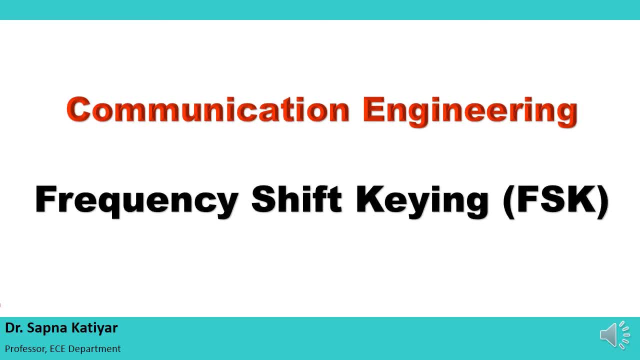 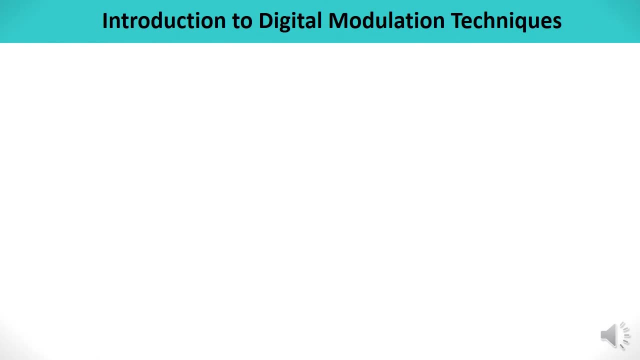 what do you understand by FSK, how to draw the FSK modulator, demodulator, and what are the various advantages, disadvantages and applications of frequency shift keying. Let us begin Before starting the FSK, just to tell you once again what is digital modulation. 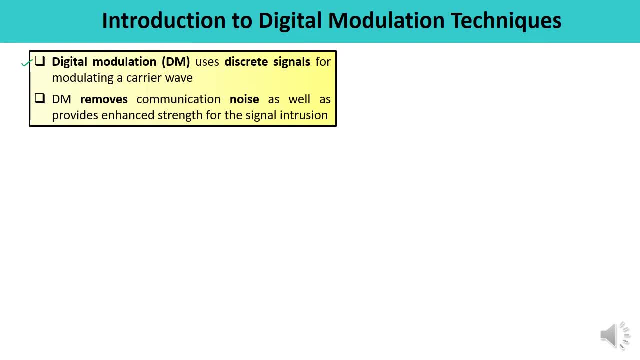 Digital modulation. it uses discrete signals for modulating a carrier. Digital modulation takes place when a carrier is modulating a carrier. Digital modulation techniques removes communication noise as well as it provides the signal strength. So there are various advantages because of which digital modulation techniques are always preferred. 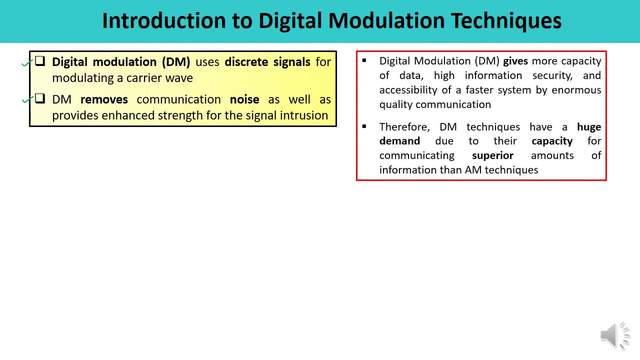 over the analog. It also gives more capacity of data, high information security, accessibility of data is being done at a faster rate and at the same time, it provides quality communication. So, because of these various impact factors, there are many very powerful factors which are giving the advantage. is digital modulation. 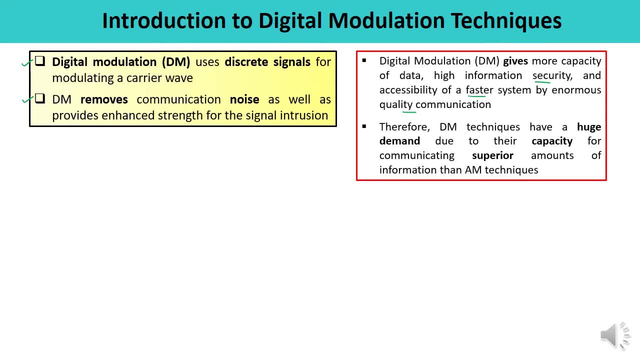 techniques are in huge demand nowadays, Especially for their capacity and for the superior amount of information if you compare with respect to the analog modulation, So it is being used frequently. There are many types of digital modulation techniques, some of the basic techniques and in some of the applications too, So these are very useful ones, For example, in In herum. 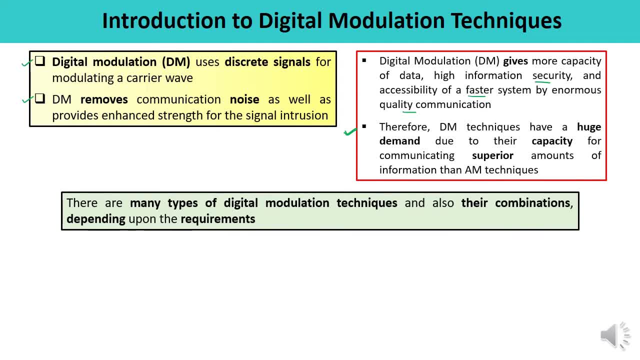 the combinations of basic techniques can also be used, depending upon the requirement. So among them, the prominent techniques are ASK, that is amplitude shift keying, FSK, which is the frequency shift keying, and PSK, which is the phase shift keying. 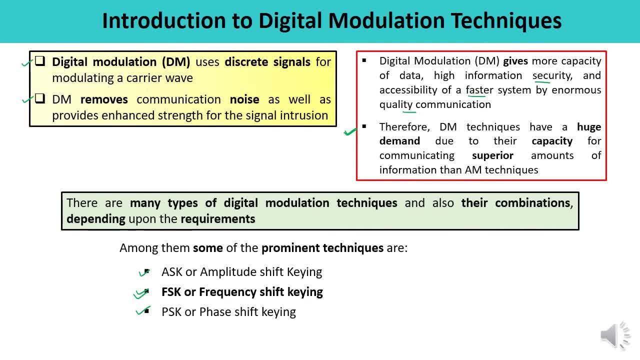 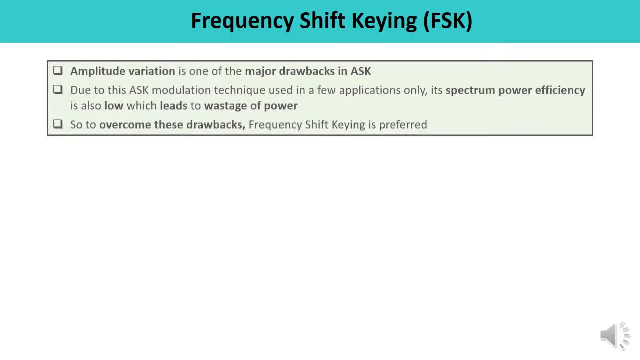 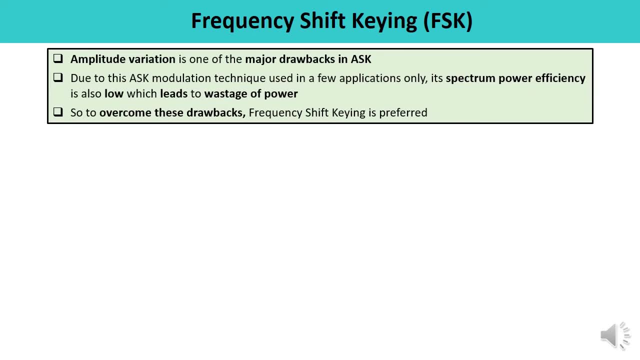 So in this video I will be talking about FSK, that is, the frequency shift keying. What is frequency shift keying and why it is used? In the previous video we have discussed about the amplitude shift keying. In case of ASK, there was a drawback, which is amplitude variation. 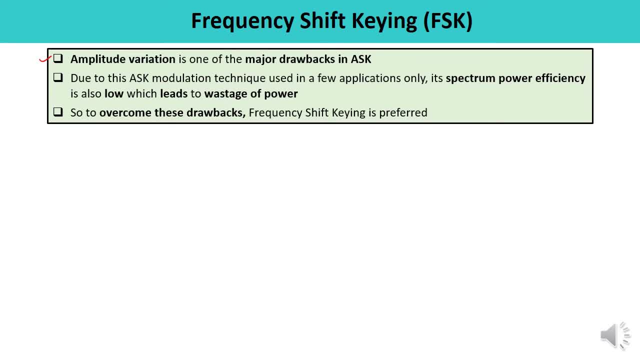 Due to this amplitude variation and there are several other factors, because it has a shortage of spectrum power efficiency and there is a power wastage also. it means all these are the drawbacks. So these drawbacks can be overcome in a technique which is known as a 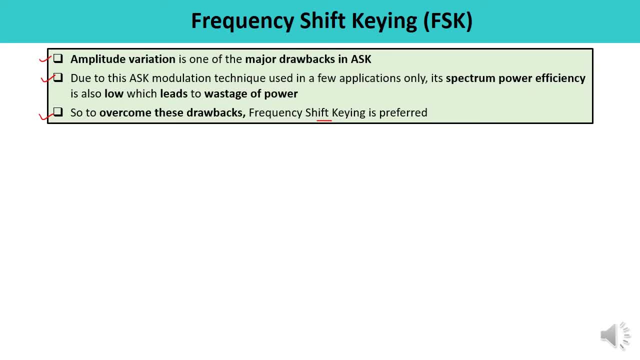 FSK, That is frequency shift keying, and because of these drawbacks only the ASK can be used into a limited number of applications. It could not be used widely. So frequency shift keying- it is the digital modulation technique in which the frequency 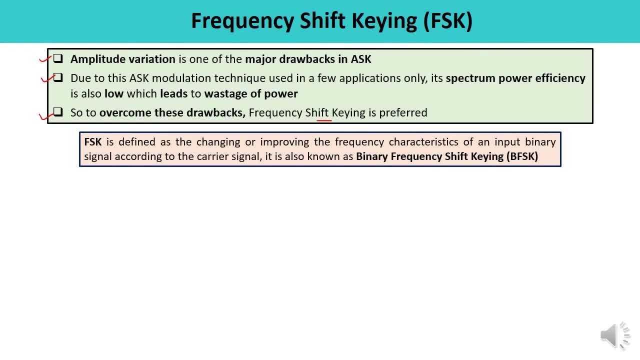 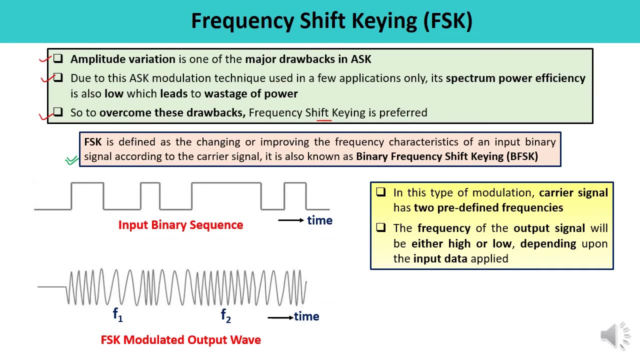 of carrier signal varies according to the digital signal changes and FSK is a scheme of frequency modulation. So what is FSK? So what happened in this particular case? in FSK there are two predefined frequencies for the carrier, as you can see in this particular diagram, two frequencies: one is F1, other is 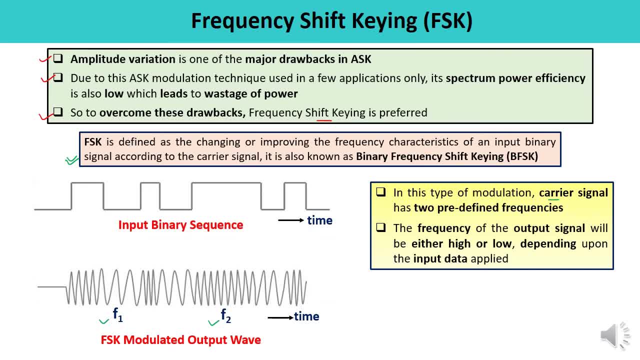 F2. Input binary sequence. definitely it must be a combination of ones and zeros. So you can observe in this particular diagram: for one there is a high frequency, for zero there is a low frequency. right, It means the output of a FSK modulation. 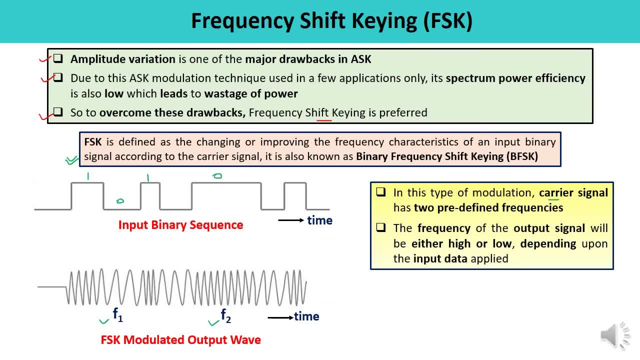 a modulated wave is high in frequency for a binary- high input. when binary input is high, that is one at the output, we will be getting high frequency and low frequency for the binary- low input here. This is one: low frequency for the binary- low input for zero. 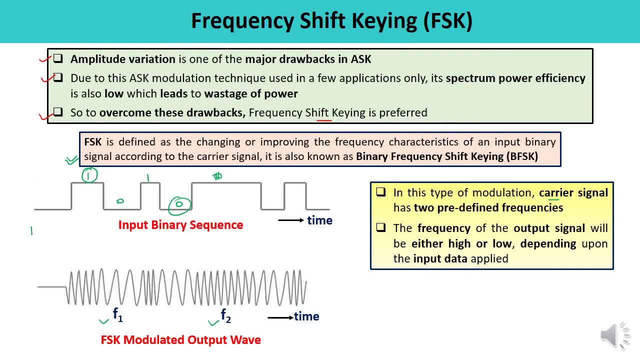 So the binary ones and zeros, they are known as mark and space. So the binary ones and zeros, they are known as mark and space respectively. for once that is mark and for zero space frequencies. so mark frequencies and space frequencies. the waveform you can see in this particular diagram, and there are various. 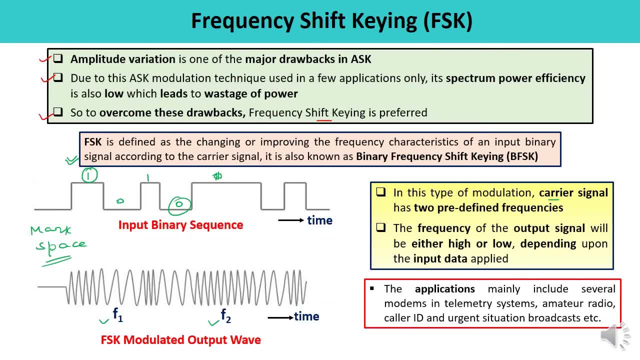 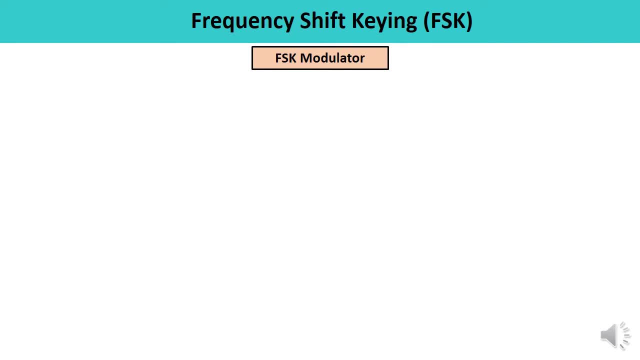 applications of FSK. it mainly includes in modems in the case of the telemetry systems, in amateur radio, caller ID in urgent situations of the broadcast. so there are various other applications also. Now let us talk about the FSK. modulator means how frequency shift keying signal is. 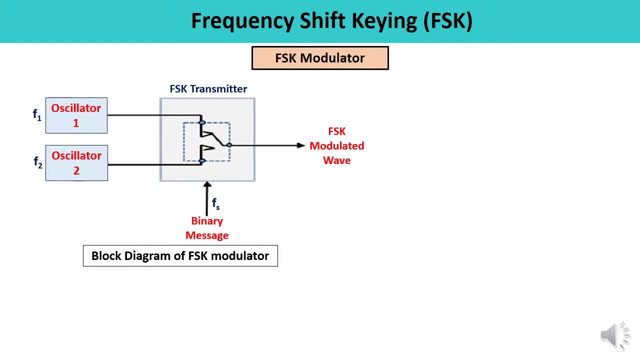 generated. so first you need to draw the diagram. you can see, this is the block diagram of FSK modulator and it consists of two oscillators, one and two, oscillator one and oscillator two, and there is an internal clock also. and one more thing: one input is the 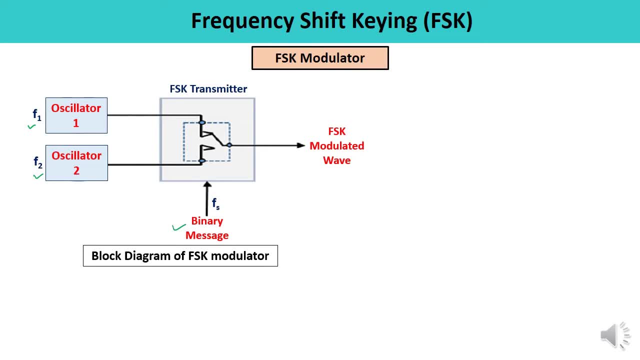 binary method, So message is in the binary form over here. So here these two oscillators- oscillator 1 and oscillator 2, they produce actually a higher and lower frequency signals. right, One will produce a higher frequency signal, or you can say one will produce a frequency F1 signal. second will produce a signal which is having a frequency F2.. 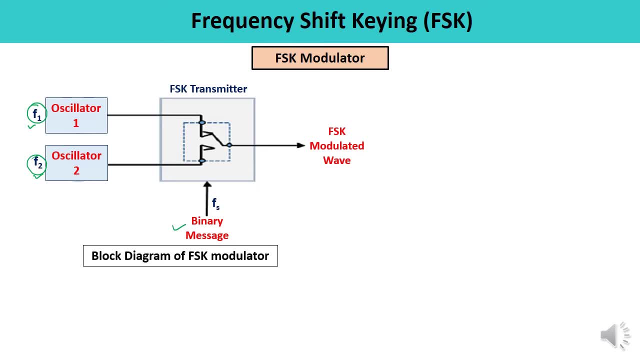 And these are connected to a switch. This is nothing but a switch, you can observe over here, along with an internal clock. Clock is internal. This is not being shown in this particular diagram, but there is a major function of the clock See to avoid the abrupt phase discontinuities of the output waveform during the transmission of the message, clock is applied to both of the oscillators. 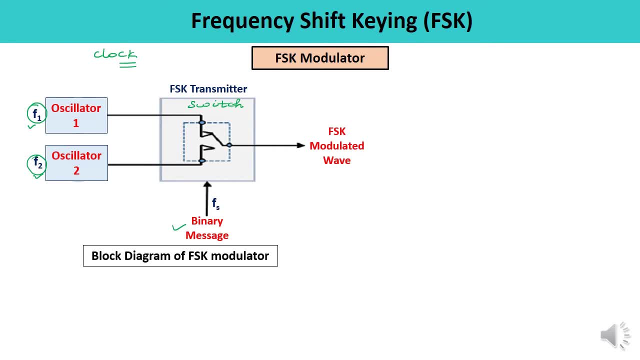 So clock is applied to both the oscillators so that phase discontinuities can be avoided. And one input to this particular block or FSK transmitter is the binary input sequence which is applied to this transmitter so that it must be capable to choose the frequencies according to the binary input. 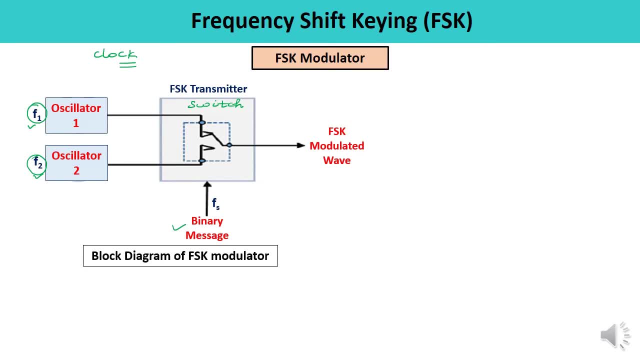 Means when the switch is closed with for oscillator 1, F1 frequency is being selected, that particular signal will be generated at the oscillator 2.. According to the binary message signal, if 0 is being applied, the switch may be moved to the oscillator 2 and that particular frequency signal may be generated. 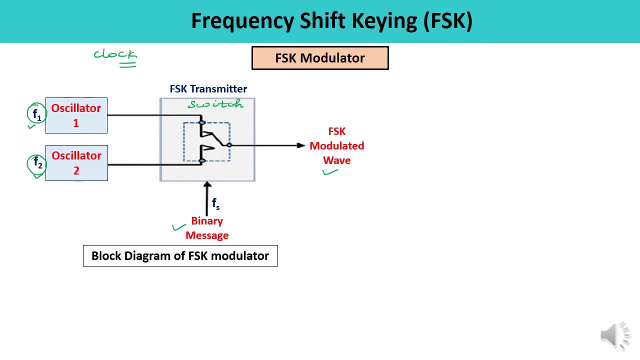 So this is how, at the output we will be getting the FSK modulated wave. You can write down the expression: if ST is the output, let us say there are two signals, M1, M2.. So it would be what? M1, T? 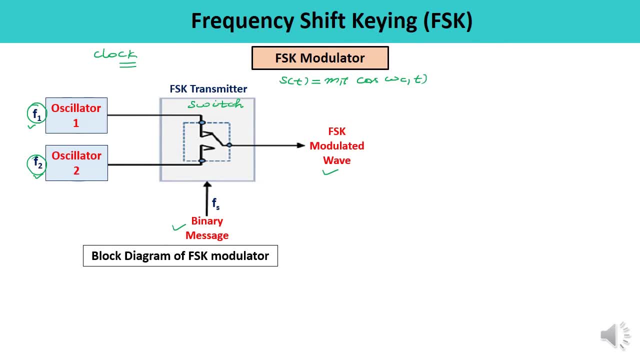 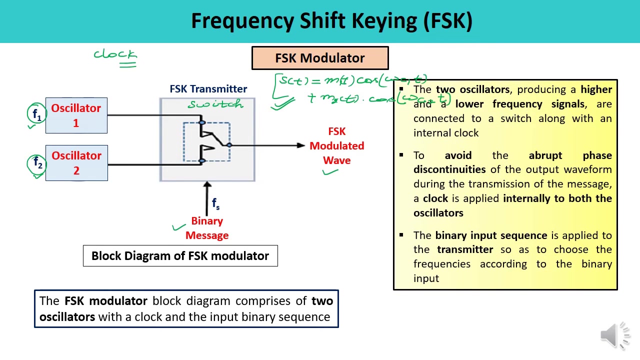 Cos omega C1 into T, plus M2T into cos omega CT C2 into T. So this is how you can write down what is the expression at the output. So the overall function which I have explained to you, I have listed out over here. 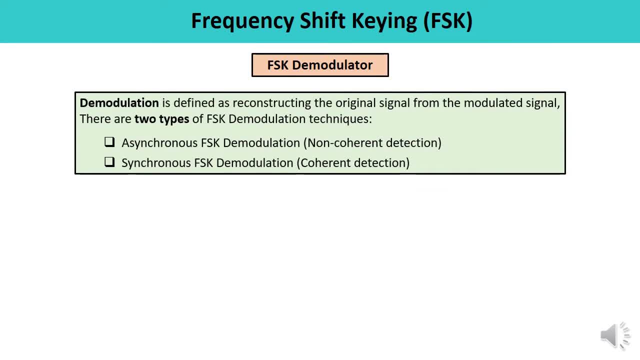 Now let us talk about the demodulator or detector. So demodulation, it is defined as the process of reconstructing original signal from the modulated signal, And there are two types of FSK demodulation techniques. One is known as a asynchronous FSK demodulation or detector. 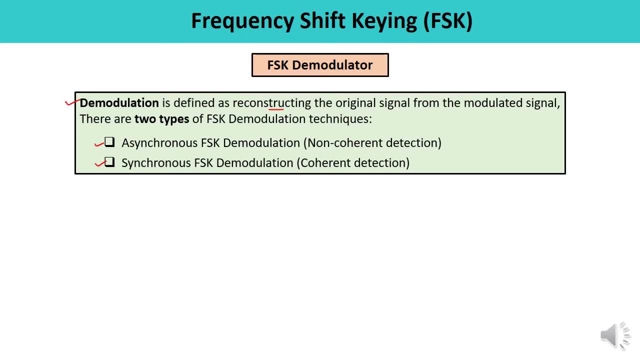 Second is synchronous FSK demodulation or detector. Asynchronous is also known as a non-coherent detection and synchronous is known as a coherent. There is a difference between the asynchronous and synchronous. In the case of the synchronous- the transmitter and receiver- they are in synchronism with the clock. 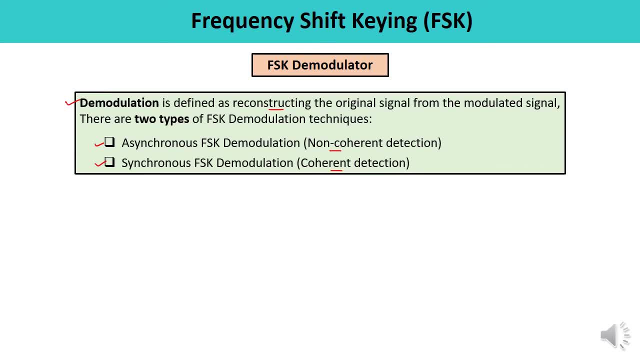 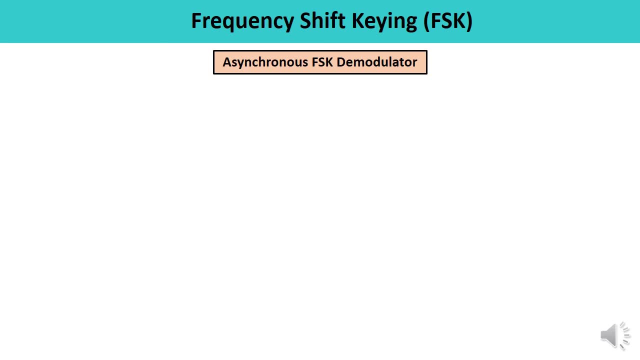 While in the case of asynchronous, there is no such type of provision. So this is how you can differentiate in between these two. Now let us talk about both of these in detail. First is the asynchronous FSK. Second is the demodulator. 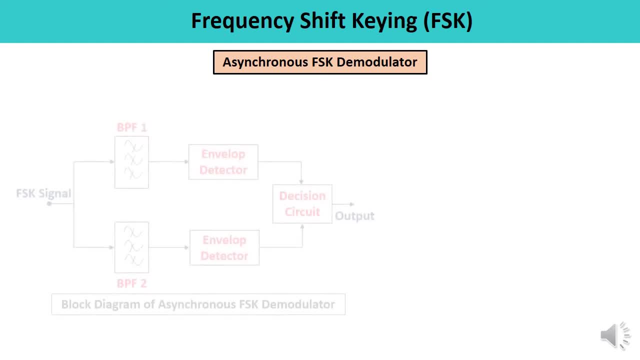 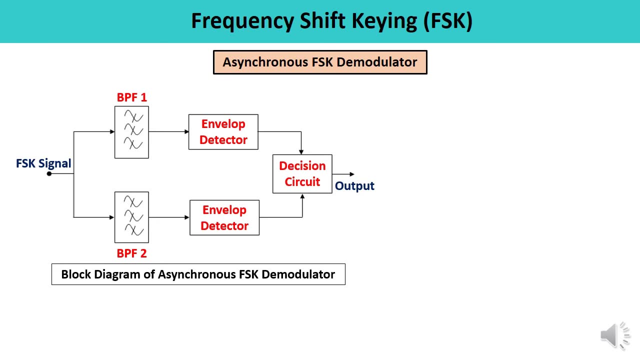 The FSK asynchronous demodulator. the block diagram you can draw in like this particular manner. This is the block diagram. Input is the FSK signal. In the previous case we have written FSK signal which we have got from the modulator, that is ST. 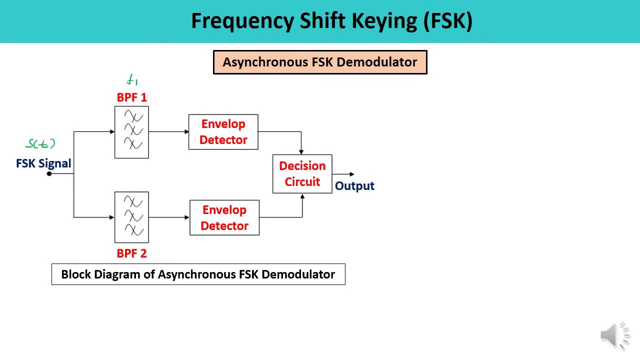 There are two bandpass filters, one and two. Let us say the frequencies which are tuned, That is, F1 and F2.. Bandpass filter 1 is tuned to frequency F1 and bandpass filter 2 is tuned to frequency F2.. 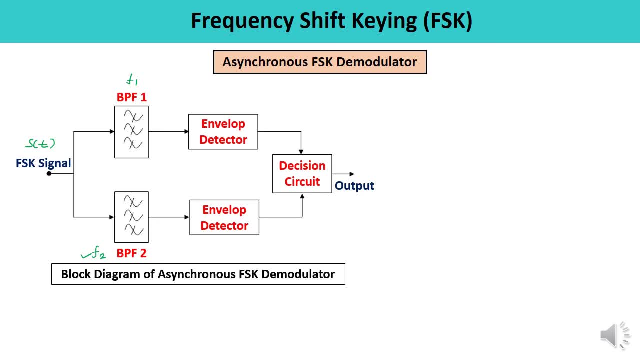 So this is how you can observe. there is a use of two envelope detectors, two bandpass filters. There is a decision circuit. What happens? The FSK signal is passed through the bandpass filter 1 and 2. Means tuned to two different frequencies, or you can say tuned to 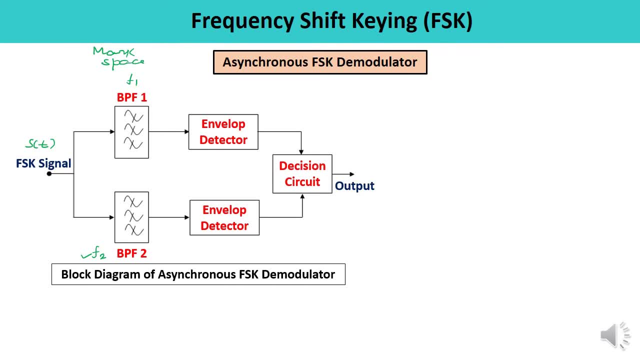 Mark and space frequencies, right. So the output from these two bandpass filters, it will looks like ASK signal. So, if you observe, the output will looks like the ASK signal Now which is being given to the envelope detector on both the sides you can see. 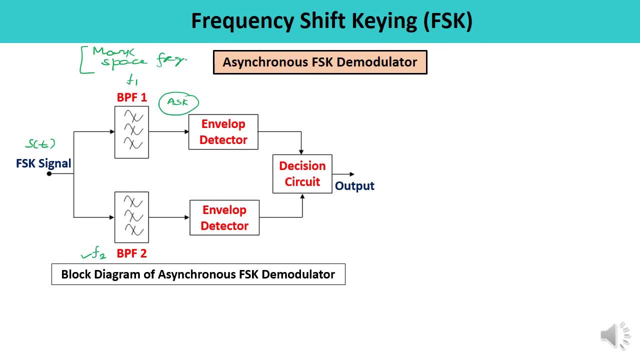 The output of bandpass filter is applied to the envelope detector And the signal in each envelope detector That is modulated asynchronously. So here the signal is modulated over here. Then you can observe there is a decision circuit. So the decision circuit actually choose which output is more likely and selected from one of the envelope detector. 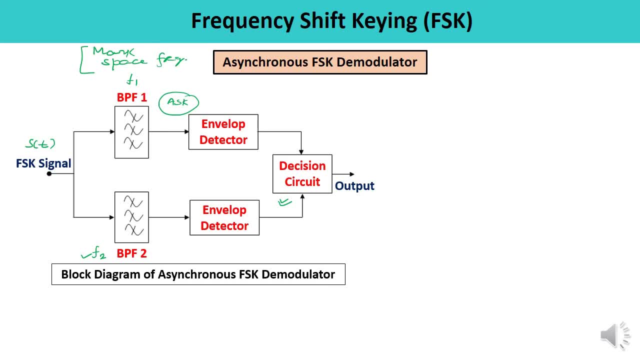 The more likely output will be selected from the envelope detector, out either from the top one or from the bottom one, And it also reshapes the waveform to a rectangle. That is why at the output again you will be getting the original signal, the message signal, that will be into the form of one or zero. 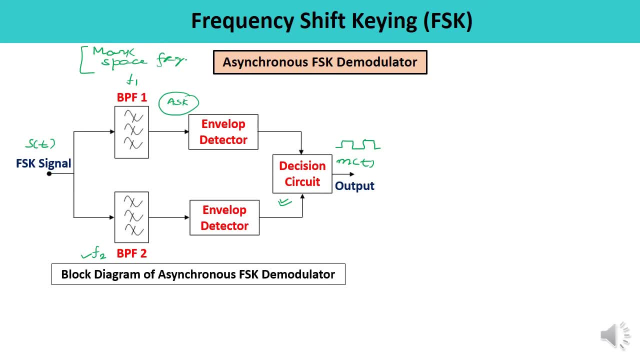 So here the important point: how the decision is being made. So a decision is made in a favor of symbol one, like how a favor is being given to the symbol one If the envelope detector output which derives from filter which is tuned to frequency F1.. 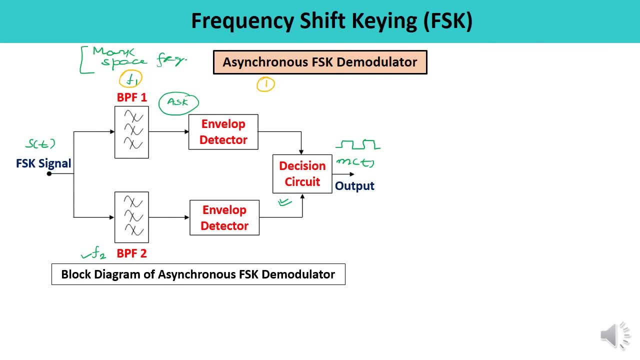 Like if this is, If the envelope detector output is tuned to frequency F1, if it is larger than the derived from the second filter. so when the frequency is larger than the derived from the second filter means output will be observed as one. otherwise a decision is will is made in favor of the zero. 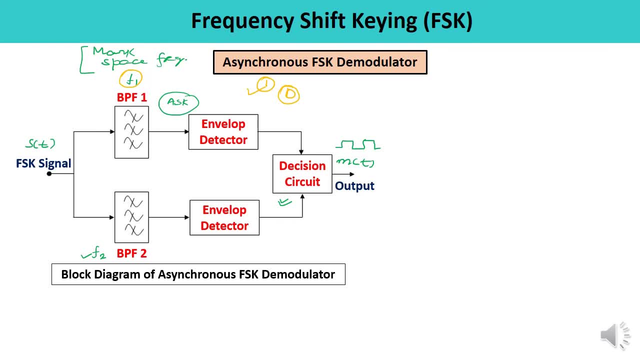 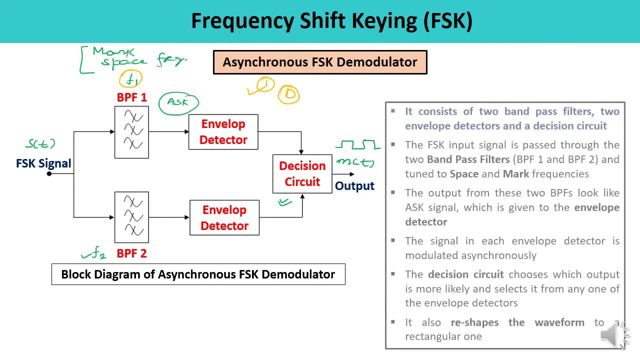 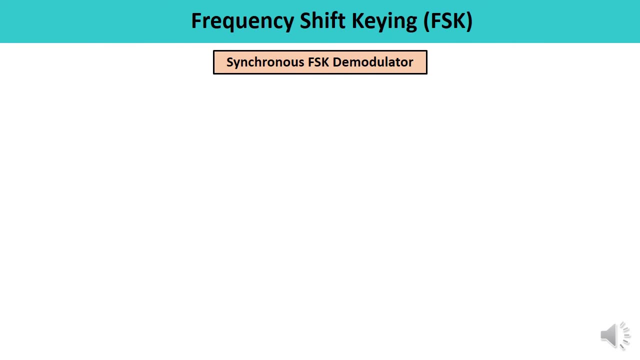 So one and zero is made, the decision accordingly, And at the output we will be getting a rectangular kind of waveform. So this is how you can explain the function of the Asynchronous FSK demodulator. Now let's talk about the synchronous FSK demodulator. 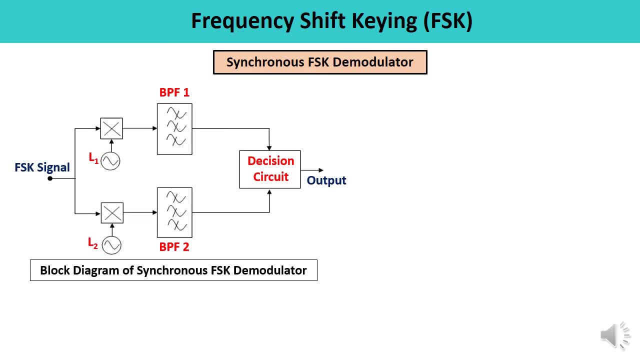 Synchronous means the coherent one. This is the block diagram for the synchronous FSK demodulator or detector. Synchronous or coherent, Coherent detection requires phase and timing synchronization. You must remember the synchronization of phase and timing. Timing is very, very required here. 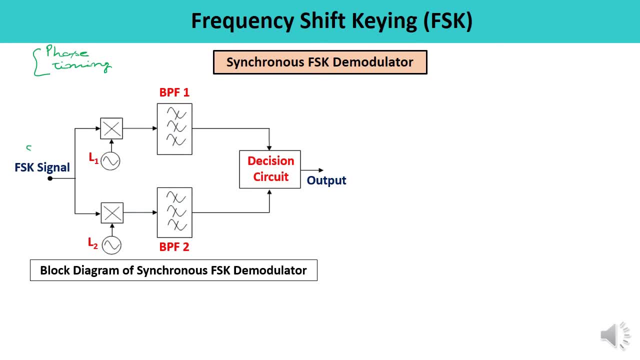 You can observe in this particular block diagram, input is the FSK signal, which is the ST, and output You require the original message signal empty, which you required at the output. And in this block diagram you can observe there are two mixers. 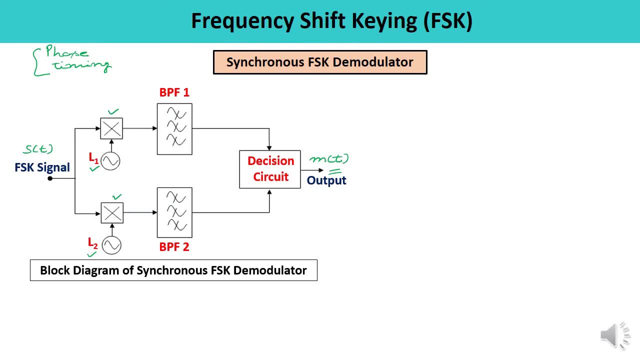 Right: Two local oscillators: local oscillators L1 and L2.. Two bandpass filters: bandpass filter 1 and 2.. And then there is a decision circuit. So this is How you can draw the block diagram. 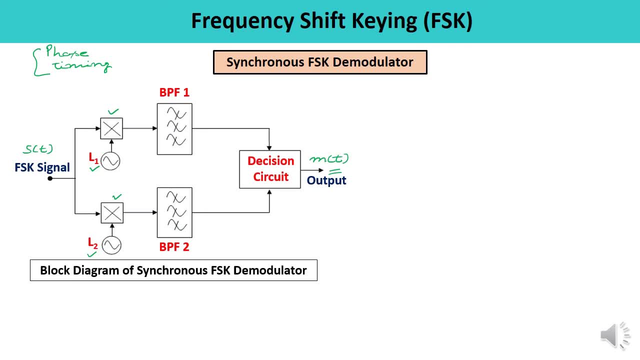 So let's start from the left hand side. The FSK signal that is given to the two mixers, mixer number one and mixer number two. So FSK signal is the input to the two mixers with the local oscillator circuits. 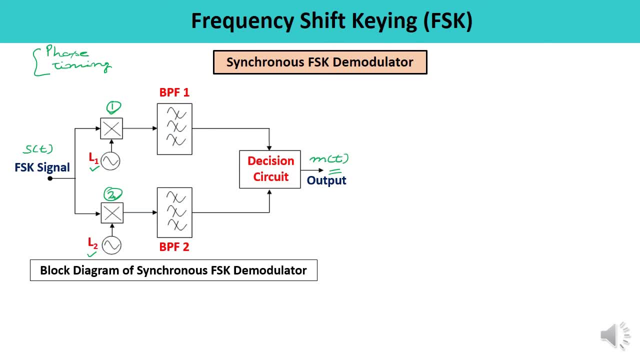 And these two are connected to the bandpass filter. So this particular combination actually acts as a demodulator Right And this is the demodulator and the decision circuit Right Which available over here. So the decision circuit choose which output is more likely and select that output from any one of the detector. output may be from at the output of bandpass filter one or from the output of the bandpass filter two. 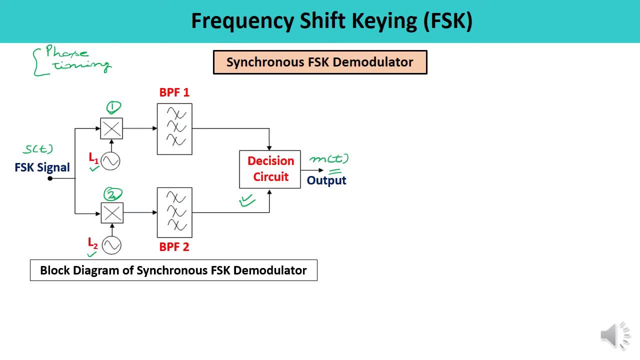 So it detects which is more likely and select accordingly. and the two signals having a minimum frequency separations. This is a required condition, So for both of the demodulator, So the bandwidth of each of them it actually depends on the bit rate. 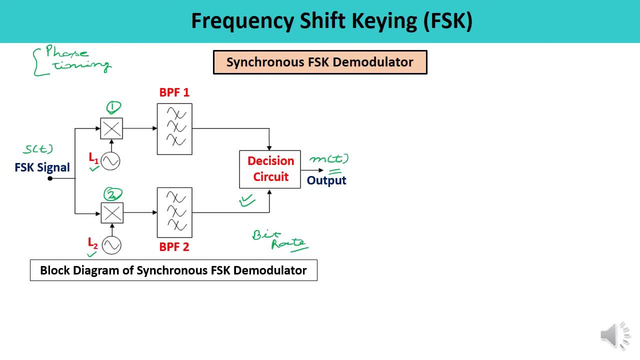 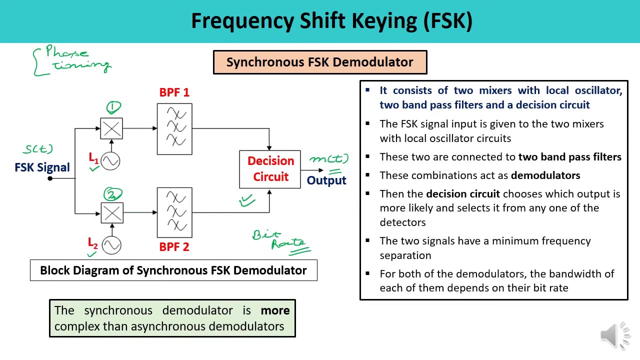 So bandwidth totally depend upon the bit rate. You must remember it, You may get a question. And the synchronous demodulator. This is a relatively complex structure in comparison to the asynchronous type demodulator. So structure is complex over here. 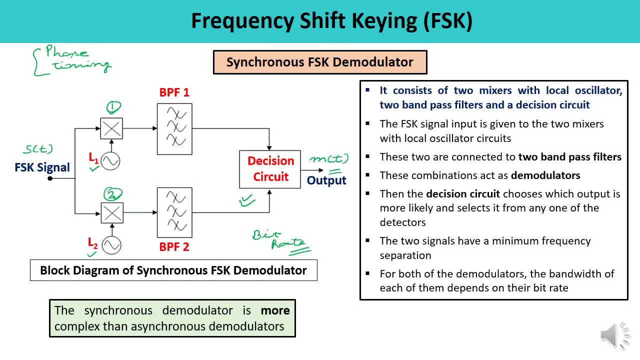 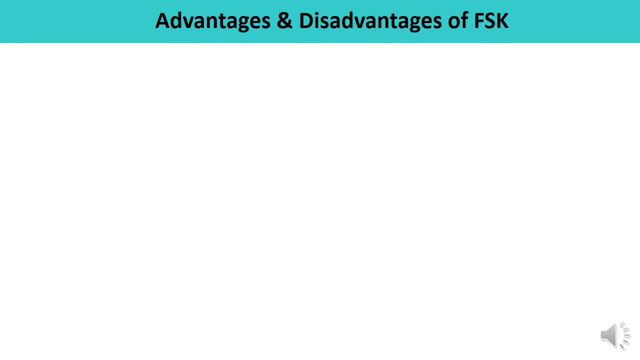 As you can observe, there is a use of two to local oscillator circuits. That is why. So this is, This is a very simple process- How the original signal, the message signal, can be reconstructed back. Now let's talk about the advantages and disadvantages of frequency shift keying. 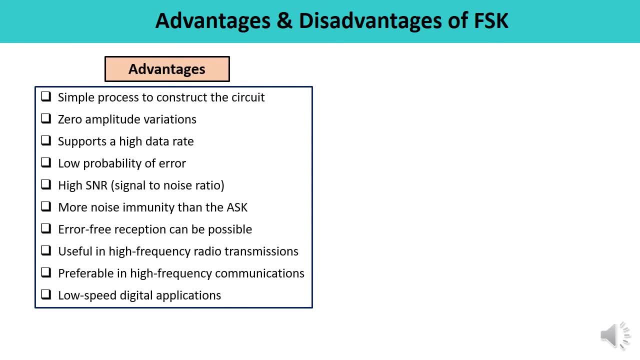 First let's talk about the advantages: Simple process to reconstruct the circuit. You have seen a very simple process for the asynchronous and even in the synchronous Also, the process is simple. Zero amplitude variation means the amplitude variation Which was the drawback of ASK that was removed over here.